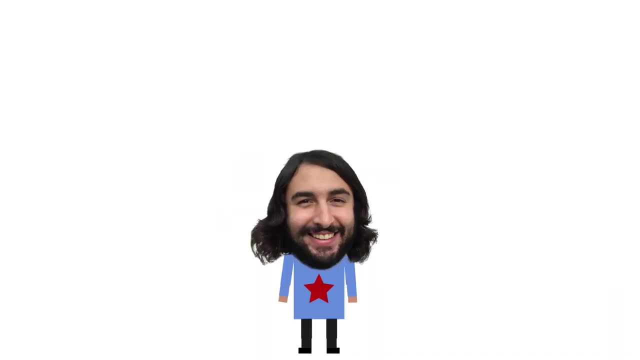 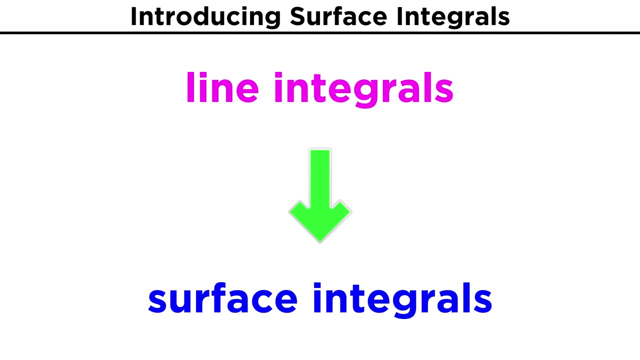 Professor Dave, here let's take a look at surface integrals. Surface integrals can be thought of as a higher dimensional equivalent to line integrals. Instead of a curve C to integrate over, we will have a surface S. If we then have a function, 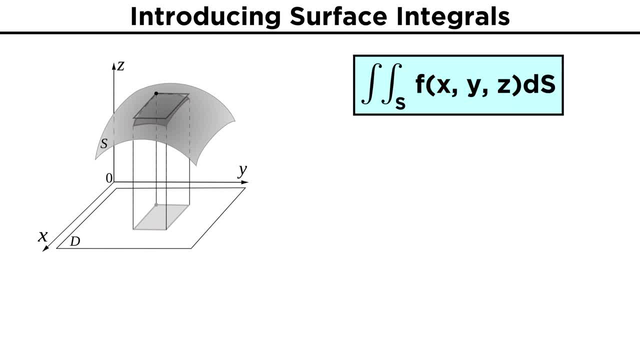 F of the surface integral of F over S will be expressed as this integral. While this expression looks fairly simple, just like constraining line integrals to the path of a curve, the complexity here comes from constraining to the surface S, And just 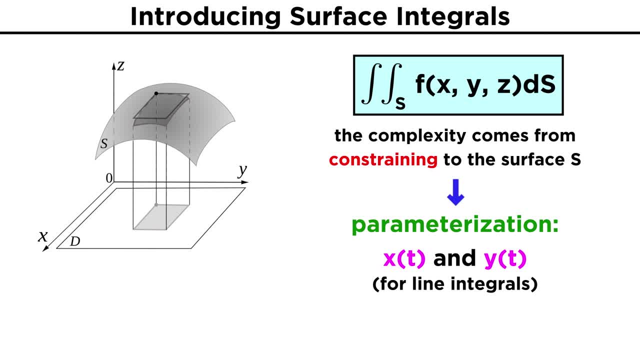 like we parameterized curves for line integrals in terms of a new variable, T, it proves useful to parameterize the surface S in terms of two new variables, Which we will call U and V. The coordinates of the surface S can be expressed as a vector. 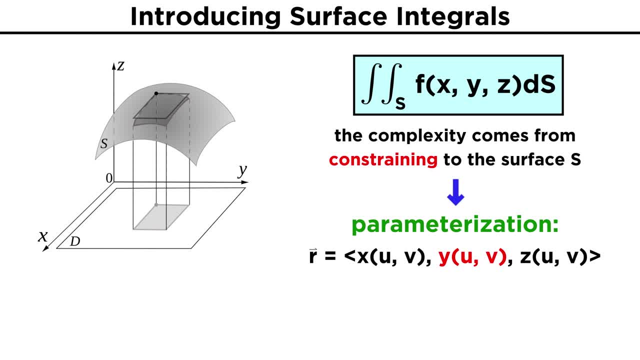 R equals X, Y, Z. With this parameterization we will be able to express the dS in the surface integral in terms we can use. It turns out that this dS can be expressed as the magnitude of the cross product of the. 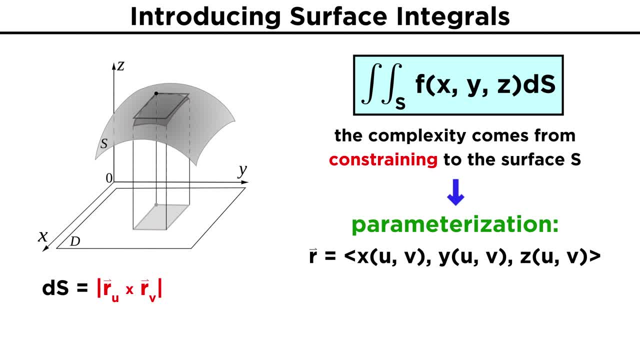 R vector's derivatives, which we will call R? U and R? V, Written out: R? U equals dX, dU, dY, dU, dZ, dU. and similarly, R? V equals dX, dV, dY, dV, dZ, dV. 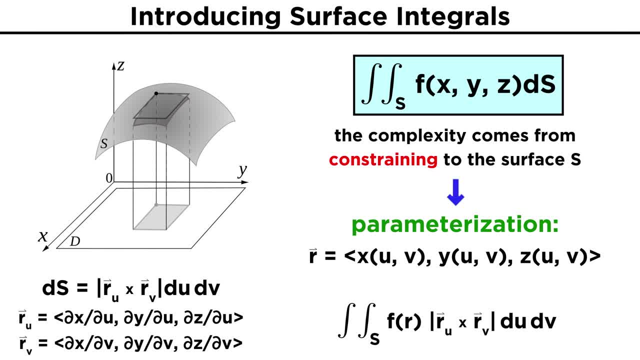 So our surface integral of F over the surface S becomes the double integral of F of R times the magnitude of R, U and R V. The interpretation of these surface integrals is a bit more abstract, but if, looking at the function, F equals one, then the integral gives back the surface area of S across the. 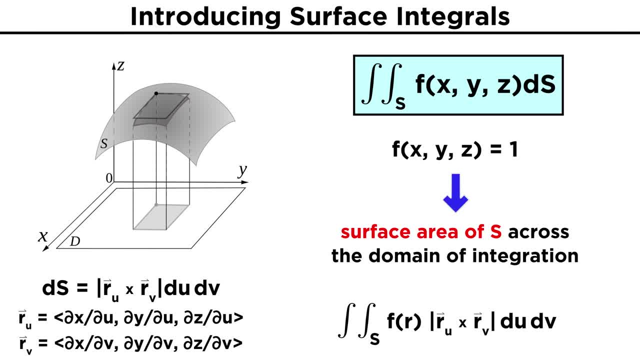 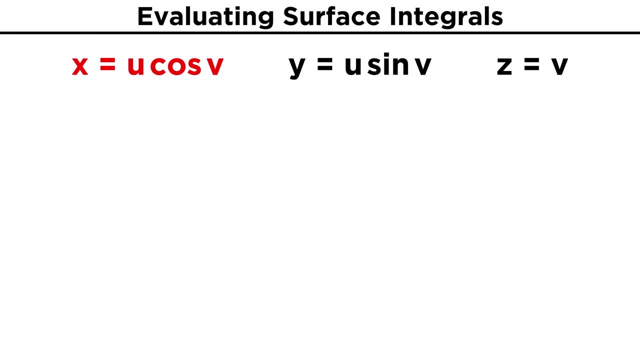 domain of the integration. For an example of how to set up the surface integral, consider the surface given by X equals U cosine V, Y equals U sine V And Z equals V. In order to set up the integral, we must take the derivatives of these expressions. 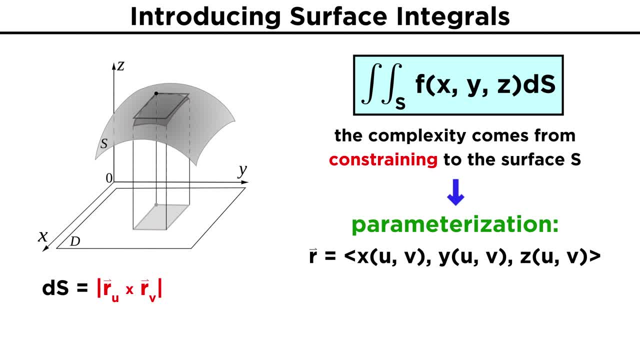 R vector's derivatives, which we will call R? U and R? V, Written out: R? U equals dX, dU, dY, dU, dZ, dU. and similarly, R? V equals dX, dV, dY, dV, dZ, dV. 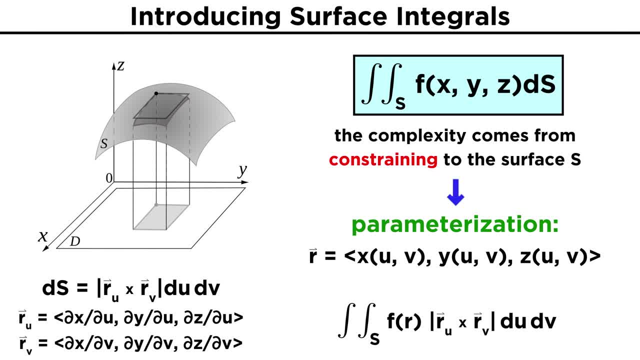 So our surface integral of F over the surface S becomes the double integral of F of R times the magnitude of R, U and R V. The interpretation of these surface integrals is a bit more abstract, but if, looking at the function, F equals one, then the integral gives back the surface area of S across the. 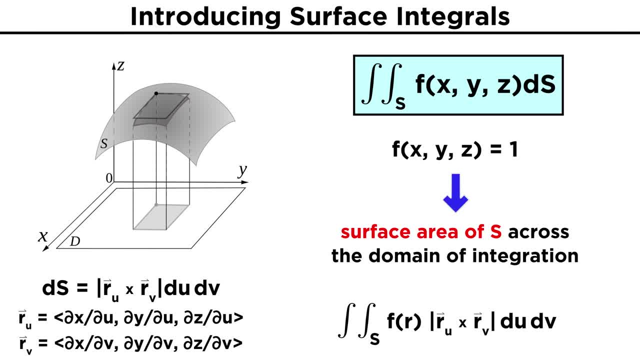 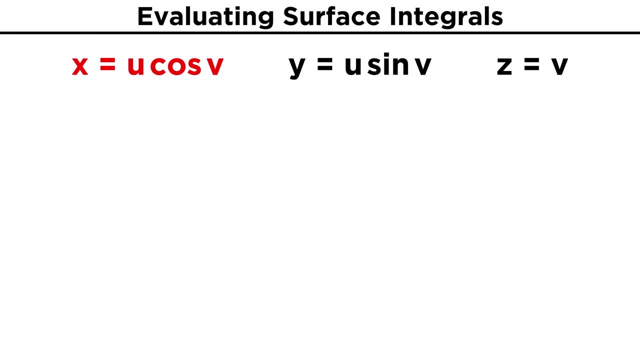 domain of the integration. For an example of how to set up the surface integral, consider the surface given by X equals U cosine V, Y equals U sine V And Z equals V. In order to set up the integral, we must take the derivatives of these expressions. 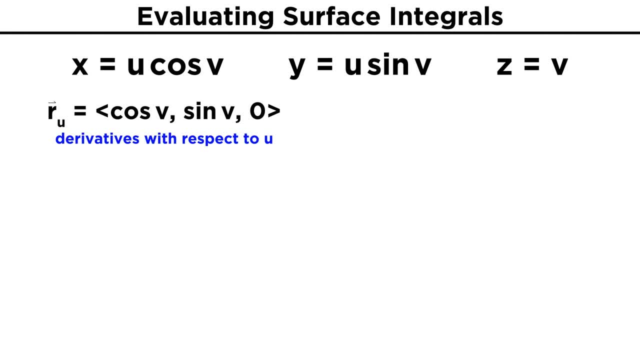 The vector R? U will be given by the derivatives with respect to U, leaving us with cosine V sine V, zero. Meanwhile, the vector R? V will be given by the derivatives with respect to V, leaving us with negative U sine V, U, cosine V and one. 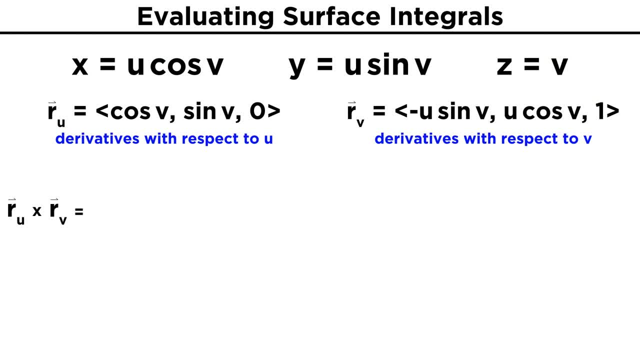 Now we must take the cross product given by R U, cross R V To find the cross product. we set up the matrix shown here and take the determinant. We end up getting sine Vi minus cosine, Vij plus U cosine squared, V plus U sine squared. 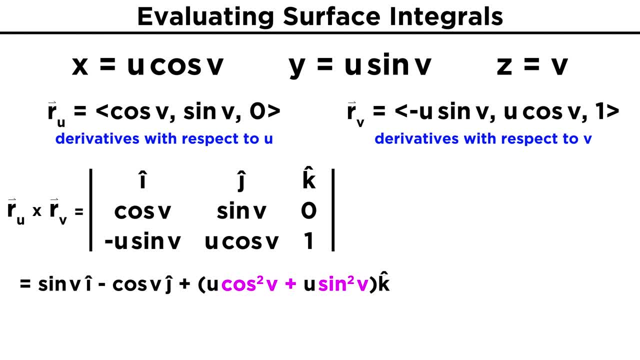 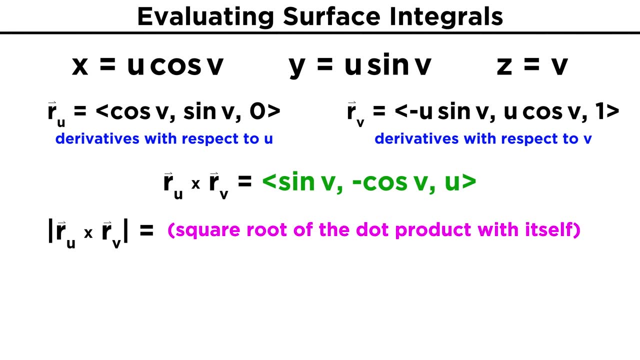 vk. And since cosine squared V plus sine squared V equals one, we end up with a vector sine squared v, with the vector sine v, negative cosine v? u. Now we need the magnitude of this vector, which, as we recall, simply means the square. 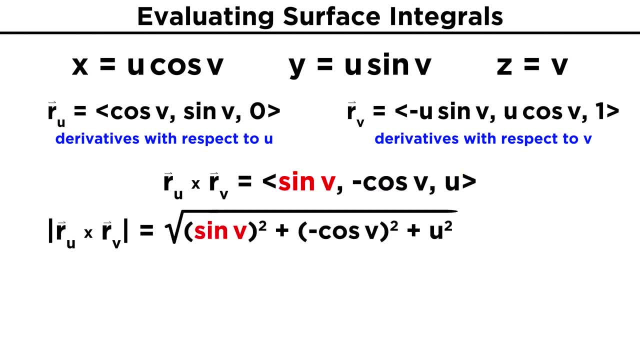 root of the dot product with itself. This gives us root sine v squared plus negative cosine v squared plus u squared, which, given the same identity we just used, becomes root one plus u squared. This is the magnitude of the cross product, making ds equal to root one plus u squared. 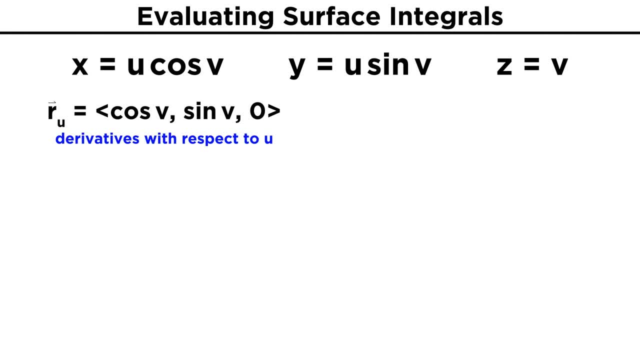 The vector R? U will be given by the derivatives with respect to U, leaving us with cosine V sine V, zero. Meanwhile, the vector R? V will be given by the derivatives with respect to V, leaving us with negative U sine V, U, cosine V and one. 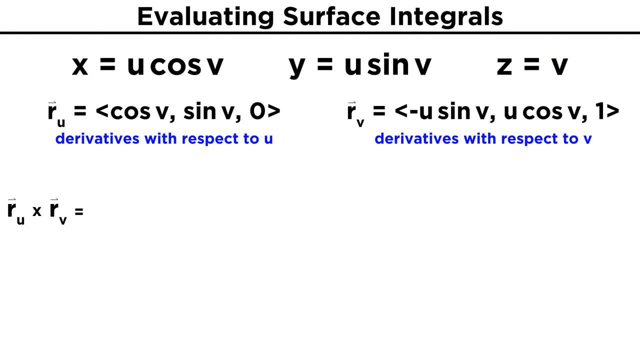 Now we must take the cross product given by R U, cross R V To find the cross product. we set up the matrix shown here and take the determinant. We end up getting sine V i minus cosine, V. j plus U cosine squared, V plus U sine squared. 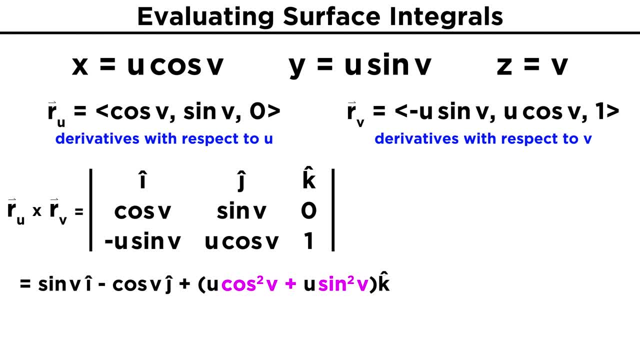 V k. And since cosine squared V plus sine squared V equals one, we end up with the vector sine V I minus cosine V j plus U sine squared V plus椩 sine squared V k. Then we have the with the vector sine v negative, cosine v u. 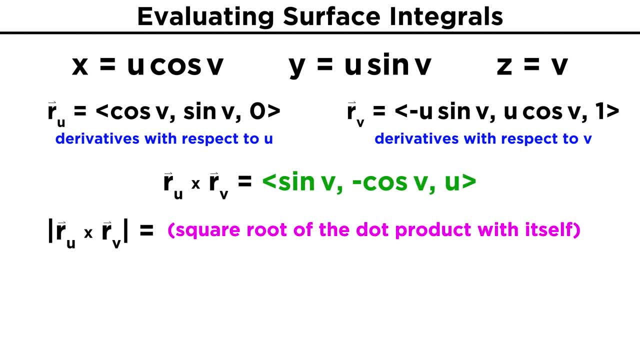 Now we need the magnitude of this vector which, as we recall, simply means the square root of the dot product. with itself, This gives us root sine v squared plus negative cosine v squared plus u squared, which, given the same identity we just used, becomes root one plus u squared. 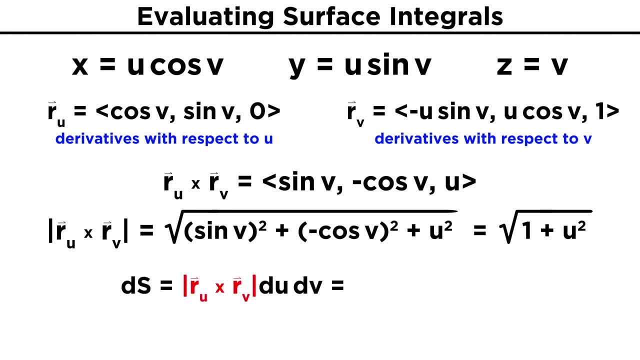 This is the magnitude of the cross product, making ds equal to root one plus u squared du dv. So our surface integral of some function, f, over this surface will be the double integral of f times root one plus u squared du dv, where f is written in terms of u and v, and 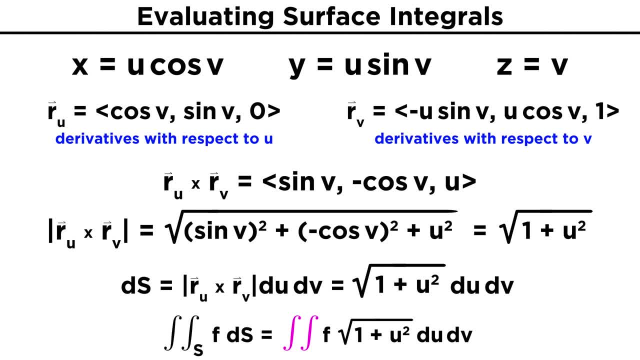 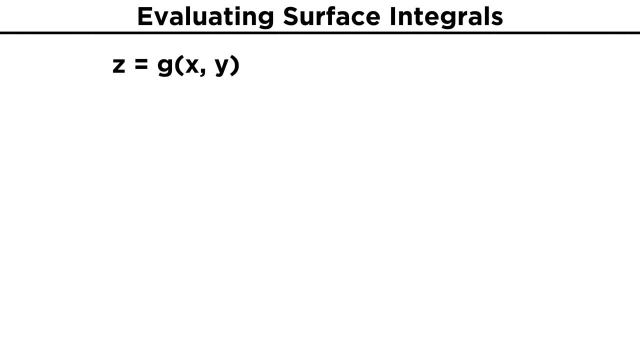 the bounds will be determined by the range of u and v. This example illustrates how to set up the most general cases of surface integrals. However, there is a simplified case where the surface we are integrating over is only a function of x and y, or in other words, z equals g of. 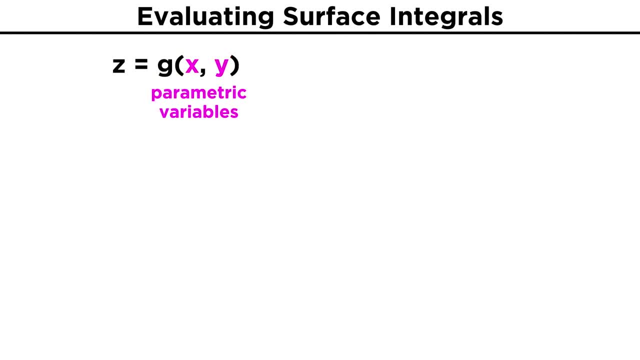 For cases like this, x and y serve as our parametric variables and our surface can be represented by the vector r equals x, y, z of. We can also use this function to calculate the function of x, y, z of. 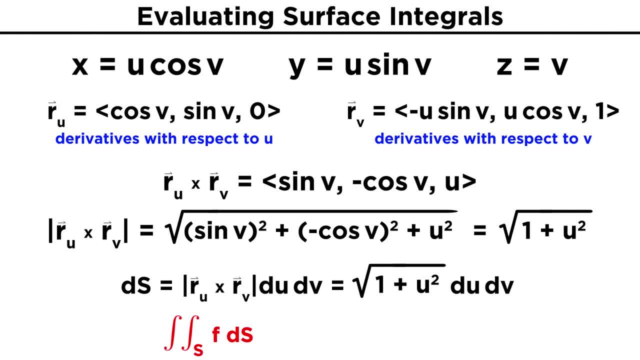 du dv. So our surface integral of some function, f over this surface, will be the double integral of f, times root one plus u squared du dv, where f is written in terms of u and v and the bounds will be determined by the range of u and v. 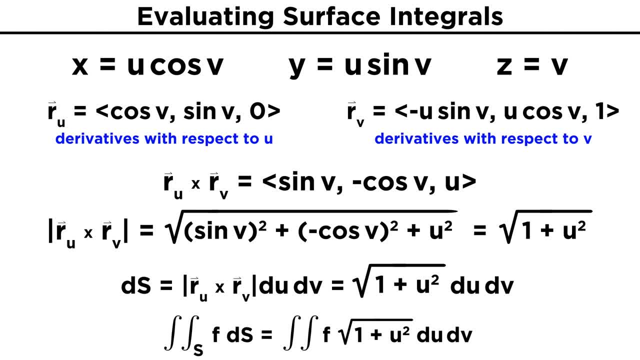 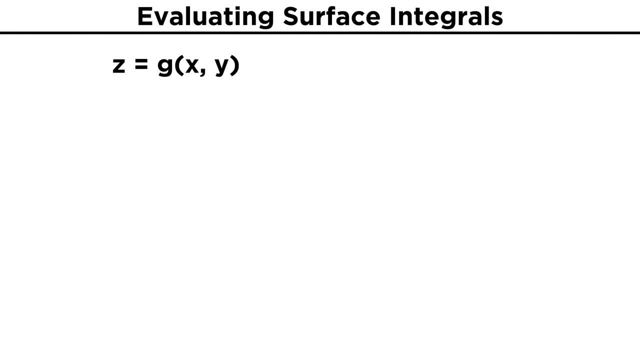 This example illustrates how to set up the most general cases of surface integrals. However, there is a simplified case where the surface we are integrating over is only a function of x and y, or in other words z equals g of. For cases like this, x and y serve as our parametric variables and our surface can. 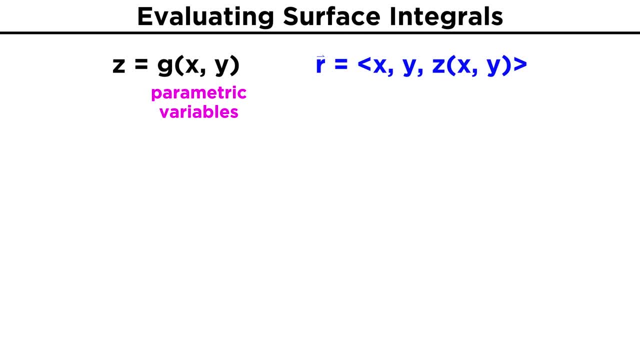 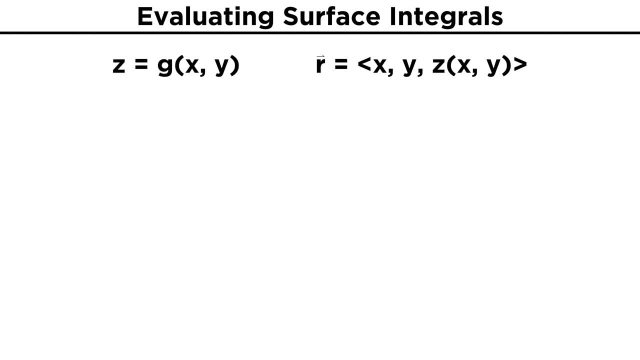 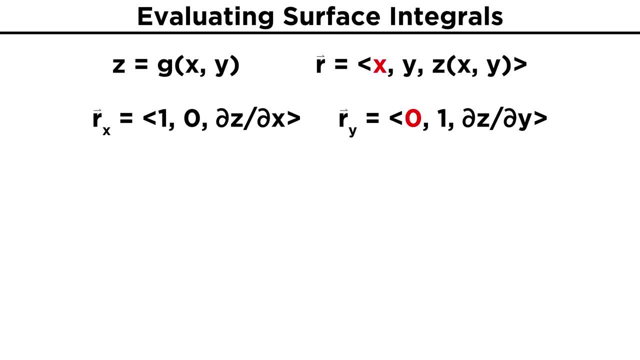 Then we find ry by taking the y derivative, giving us zero one dz dy. Now, taking the cross product rx, cross ry, we take the determinant of this matrix. We end up getting negative dz dx i. Next, we need the magnitude of this cross product, which is the square root of dz dx squared. 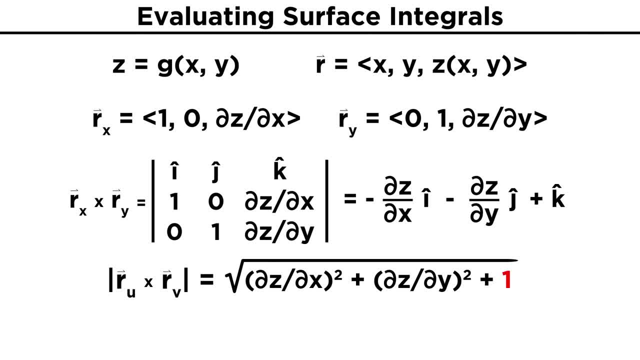 plus dz dy squared plus one. Now that we have this, we see that ds in this special case is root dz, dx squared plus dz dy squared plus one dx dy. Putting everything together, our surface integral becomes the double integral of the. 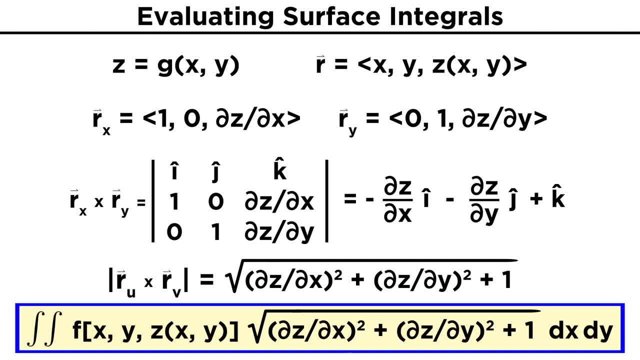 function f times root: dz dx squared plus dz. dy squared plus one dx dy. Calculations for this scenario are much more simple and follow this easy-to-calculate expression. We only need to take care when dealing with complex bounds for x and y. 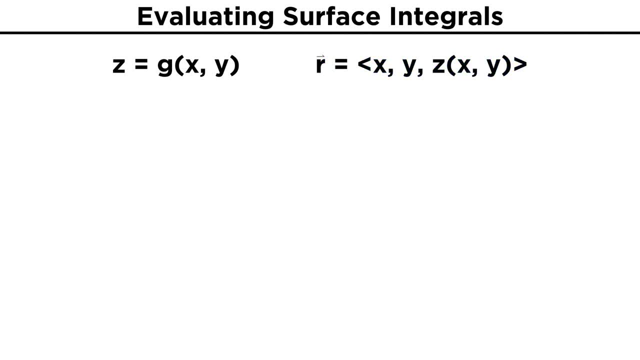 For cases like this, x and y serve as our parametric variables and our surface can be represented by the vector r equals x, y, z, of. Let's find the expression for ds in this case. First we find the vector rx by taking the x derivative, giving us one zero, dz, dx. 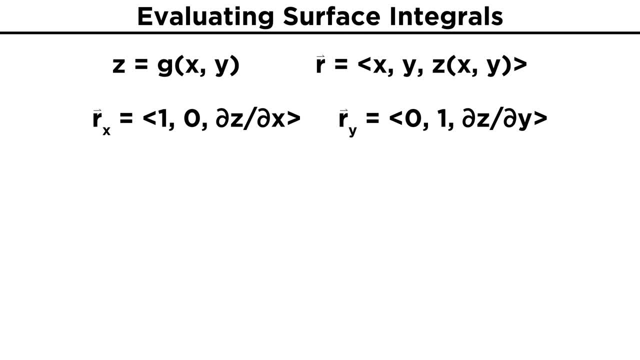 Then we find ry by taking the y derivative, giving us zero one dz dy. Now, taking the cross product, rx, cross ry, we take the determinant of this matrix. We end up getting negative dz dx i. We end up getting negative dy i minus dz dy j plus k. 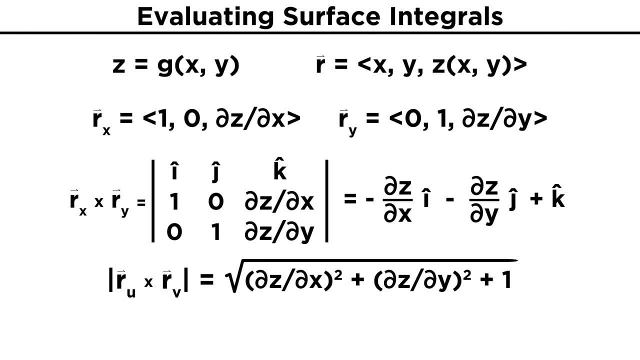 Next, we need the magnitude of this cross product, which is the square root of dz. dx squared plus dz. dy squared plus one. Now that we have this, we see that ds, in this special case, is root, dz dx squared plus. 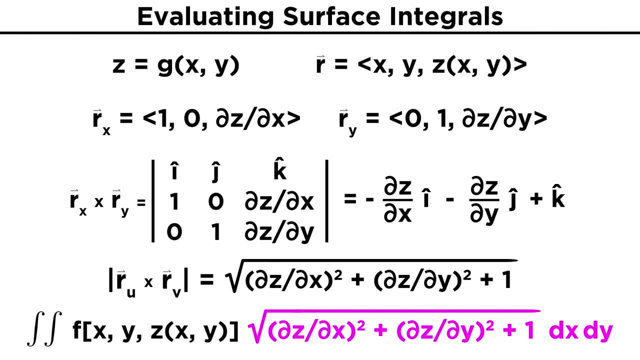 dz dy squared plus one dx dy. Putting everything together, our surface integral becomes the double integral of the function f times root: dz dx squared plus dz dy squared plus one dx dy. Calculations for this scenario are much more simple and follow this easy to calculate expression: 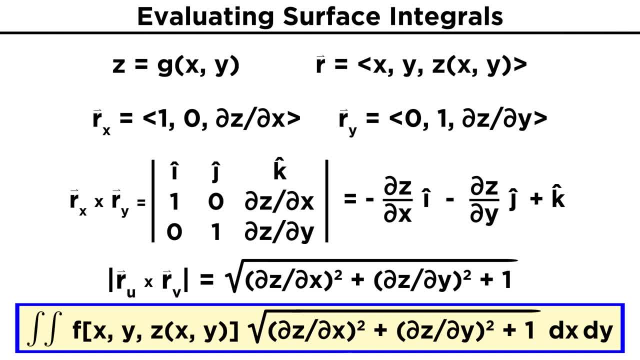 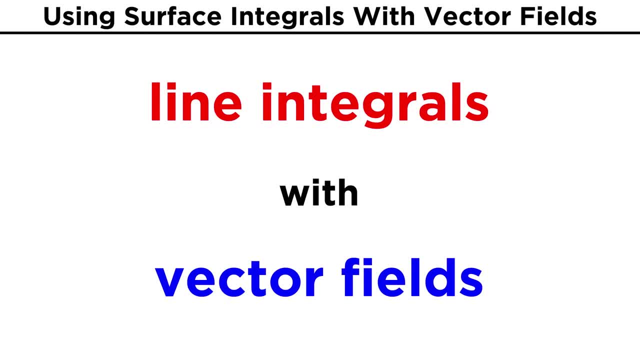 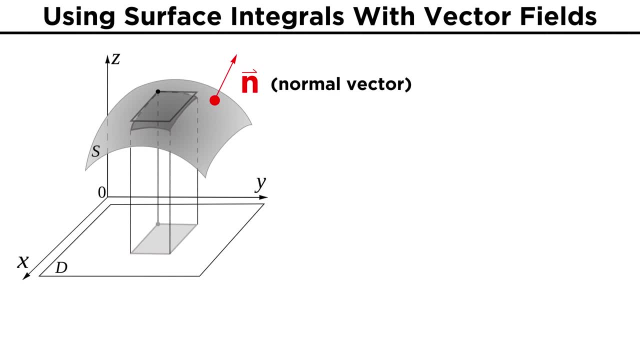 We only need to take care when dealing with complex bounds for x and y. Finally, just the way that line integrals could be used with vector fields. surface integrals can do the same. In order to express surface integrals with vector fields, we must first introduce the 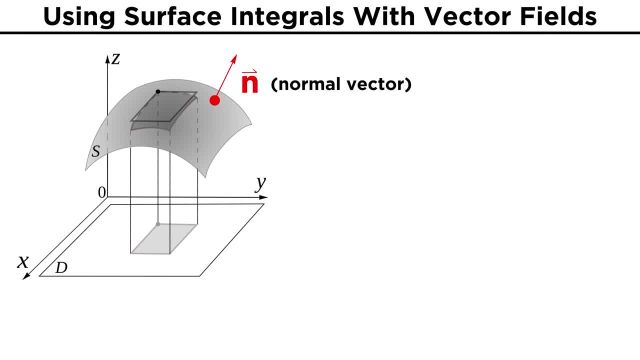 normal vector n. If we have a surface to integrate over, the normal vectors at each point are unit vectors that point in perpendicular fashion away from the surface. An easy way to visualize this would be to imagine running a flat piece of paper on the. 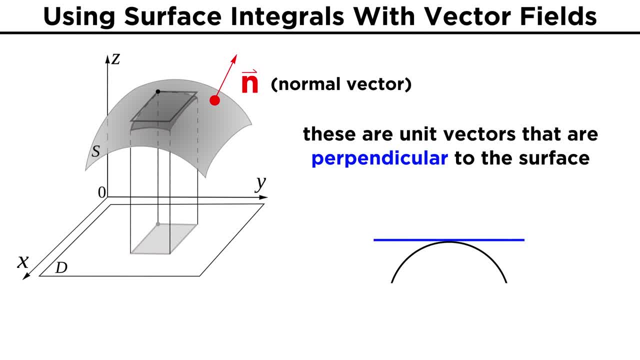 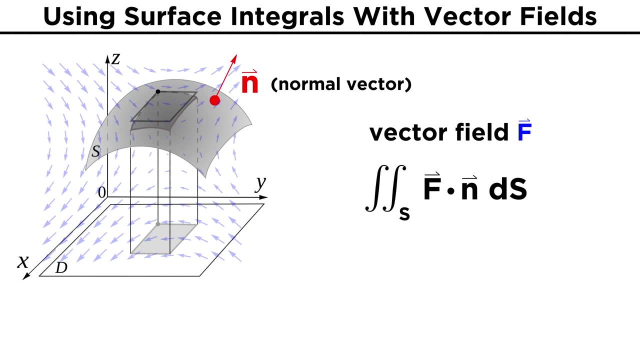 surface. The direction straight out of the paper is the normal vector. Now, if we have a vector field f permeating space, the surface integral of f over the surface s will be f dot, the normal vector n ds. This calculation ends up describing the amount of the vector field f that passes through. 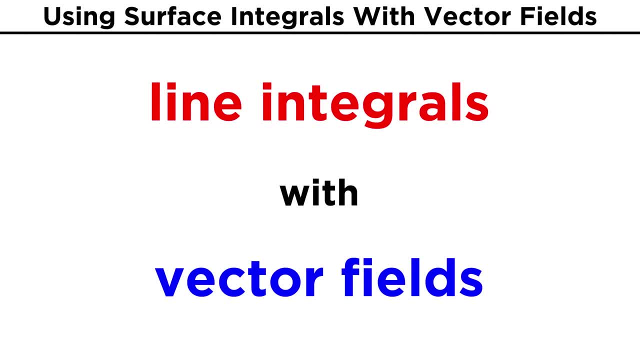 Finally, we can use this equation to calculate the function of x, y, z of. We can also use this equation to calculate the function of x, y, dx, dy. Finally, just the way that line integrals could be used with vector fields surface. 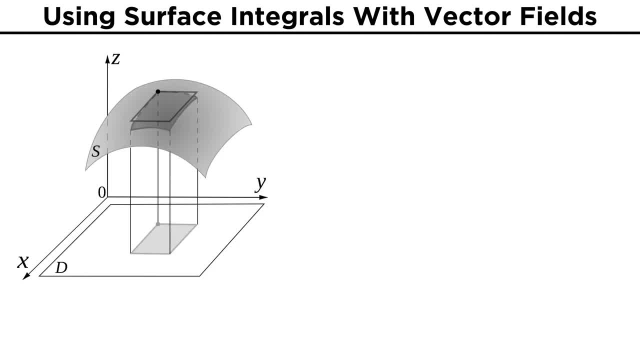 integrals can do the same. In order to express surface integrals with vector fields, we must first introduce the normal vector n. If we have a surface to integrate over the normal vectors at each point are unit vectors that point in perpendicular fashion away from the surface. 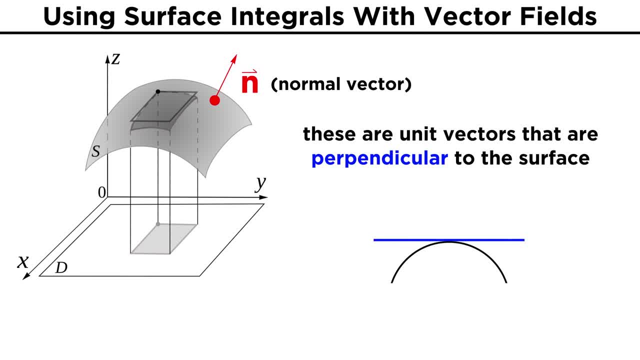 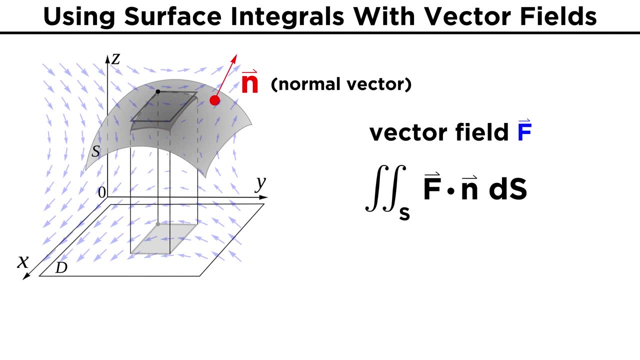 An easy way to visualize this would be to imagine running a flat piece of paper. The direction straight out of the paper is the normal vector. Now if we have a vector field, f, permeating space, the surface integral of f over the surface s will be f, dot the normal vector n, ds. 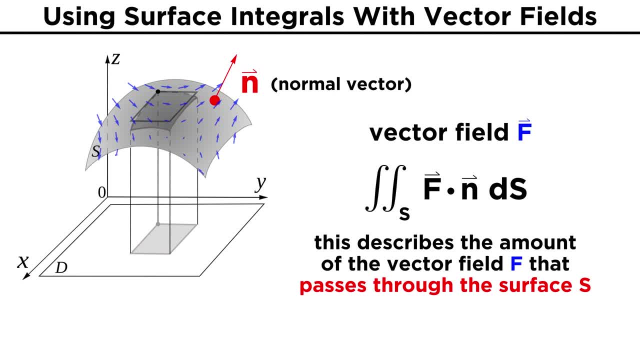 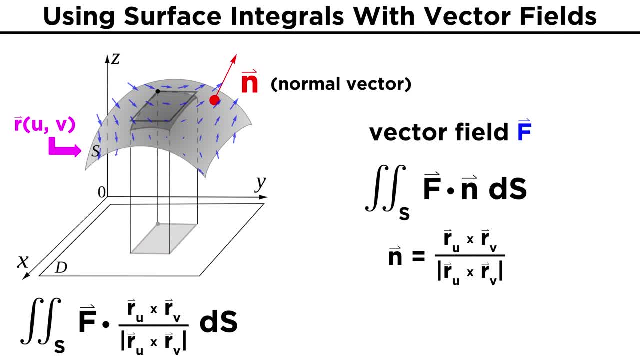 becomes F dot R? U cross R V divided by the magnitude of that cross product D S. But recall that D S equals the magnitude of the cross product times D U D V. Plugging this in cancels the magnitudes out, leaving us with the double integral F dot R U cross R. 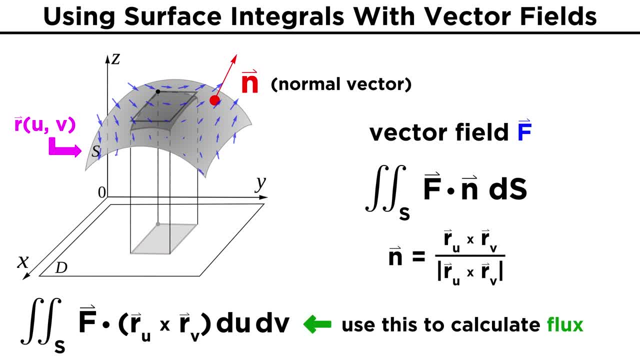 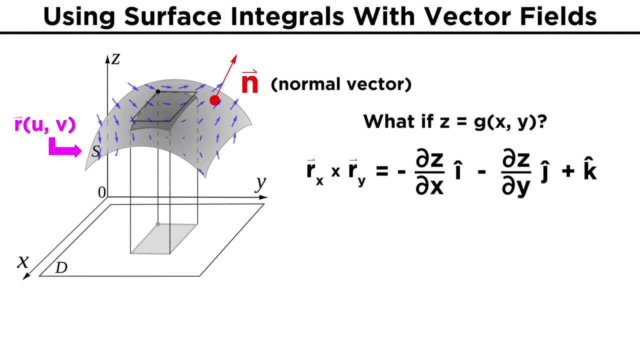 V, D U D V. This is the expression we can use to calculate the flux in any general case. but let's once again consider a surface where Z is a function of X and Y. We saw in this case that R X cross, R Y equals negative D, Z, D, X, I minus. 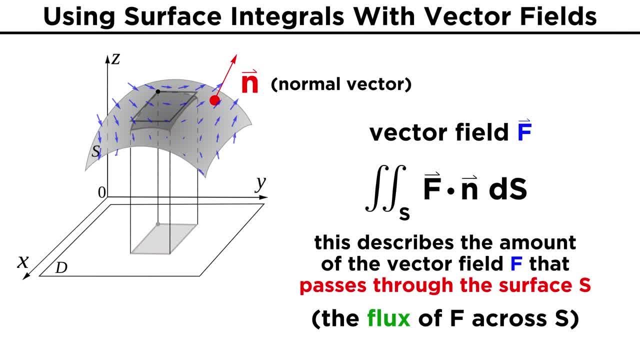 the surface s also called the flux. In order to go through calculations, we must know how to express the normal vector in terms we can use For surfaces that are given by a parameterized r of uv vector, like we discussed earlier. the n vector ends up being equal to ru cross rv divided by the magnitude of ru cross rv. 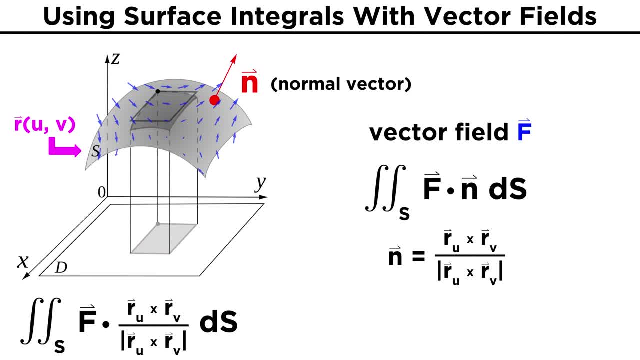 So our surface integral becomes f dot uv. We can also use the f dot ru cross rv divided by the magnitude of that cross product ds. But recall that ds equals the magnitude of the cross product times du dv. Plugging this in cancels the magnitudes out, leaving us with the double integral f dot. 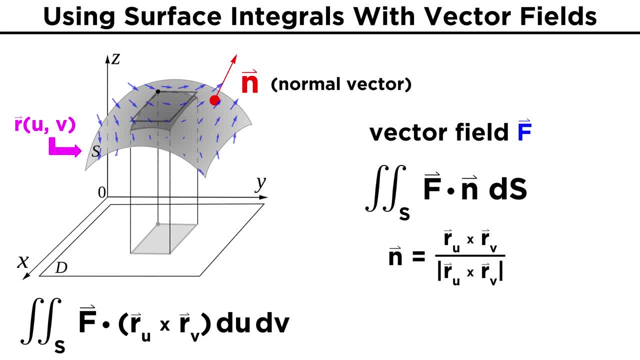 ru cross rv, du dv. This is the expression we can use to calculate the flux in any general equation, general case. but let's once again consider a surface where z is a function of x and y. We saw in this case that rx cross ry equals negative dzdxi minus dzdyj plus k. 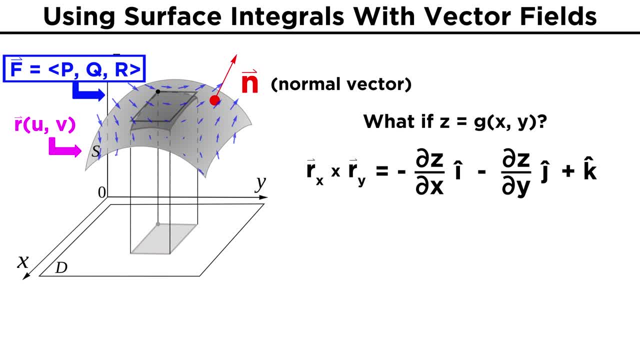 Recall how we can write vector fields in components p, q, r, so the dot product f, dot, rx, cross ry ends up being negative, p, dzdx minus q, dzdy plus r, And so in this case our flux becomes the double integral of this expression: dxdy. 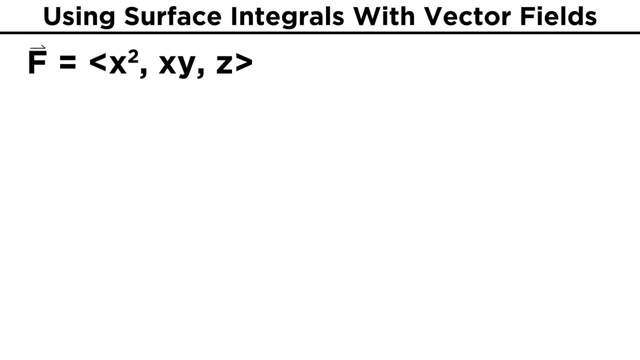 For a complete example, consider the vector field: f equals x squared, xy z, and the surface given by z equals x plus y squared. Let's think about this. Let's find the flux of the field through this surface over the range x, from zero to. 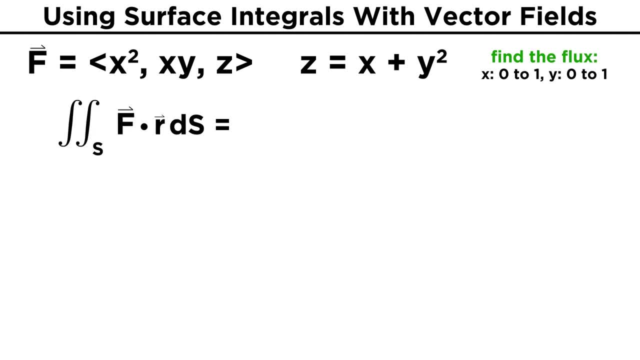 one and y from zero to one. Since the surface is given as a function of x and y, we can jump to expressing our surface integral as the double integral of negative p, dzdx minus q, dzdy plus r, dxdy. Here p is x squared and dzdx is the x derivative. 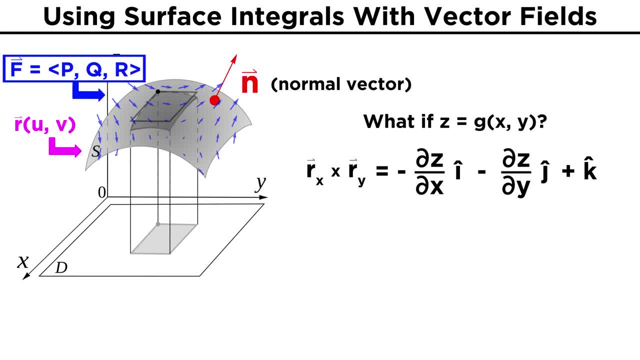 D, Z, D, Y, J plus K. Recall how we can write vector fields in components P, Q, R. so the dot product F, dot, R, X, cross, R, Y ends up being negative: P, D, Y, J plus K, And so in this case our flux becomes the double integral of this expression: D X, D, Y. 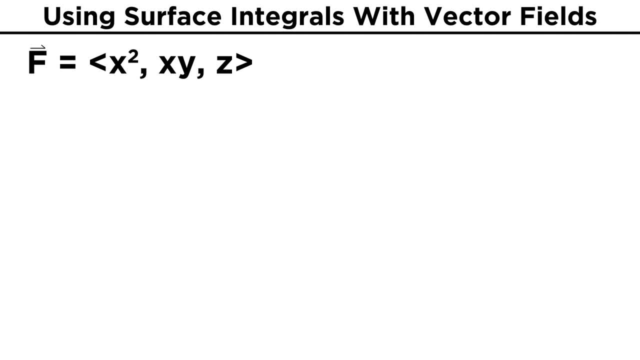 For a complete example, consider the vector field: F equals X squared, X, Y, Z, and the surface given by Z equals X plus Y squared. Let's find the flux of the field through this surface over the range X from zero to one and Y from zero to one. 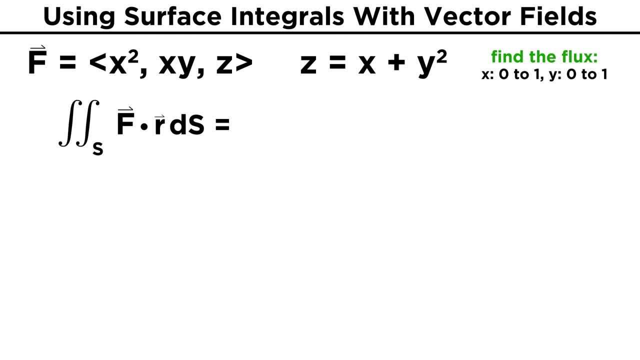 Since the surface is given as a function of X and Y, we can jump to expressing our surface integral as the double integral of negative P D Z D X minus Q D Z D Y plus R D X, D Y. Here P is X squared and D Z D X is the X derivative of X plus Y squared, which equals: 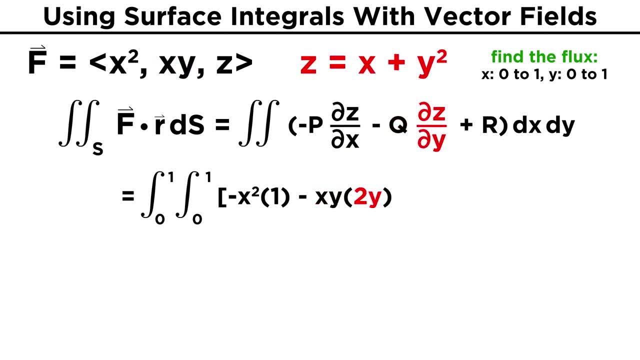 one Q is xy and dzdy will be the y derivative of x plus y squared. so two y And r is z, which, in terms of x and y, is x plus y squared. Plugging all this in we get the double integral. 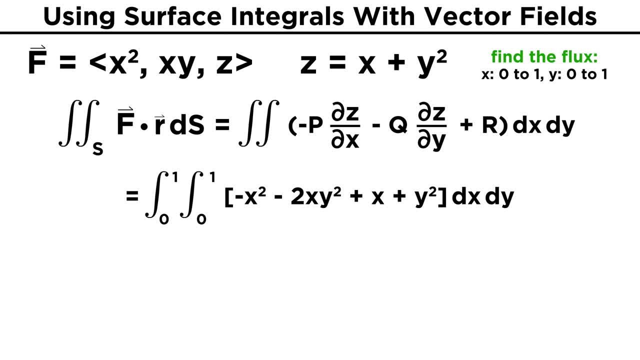 of negative x squared minus two, xy squared plus x plus y squared dxdy, where both x and y range from zero to one. Evaluating the x integral first, we get the antiderivative negative x cubed over three minus x squared y squared plus x squared over two plus xy. 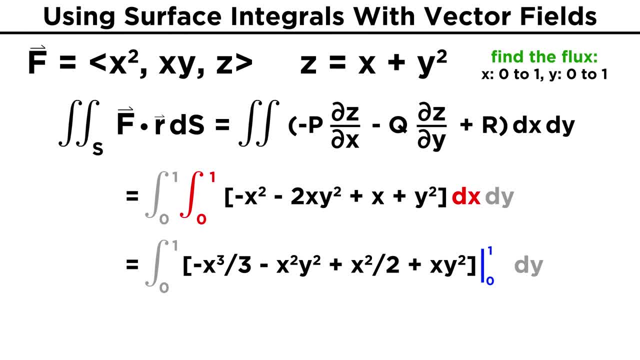 squared where x runs from zero to one. Evaluating at x equals one gives negative. one third minus y squared, plus one half plus y squared, while evaluating at zero will just give zero. The y squared terms cancel, leaving us with the integral from zero to one of one. sixth, 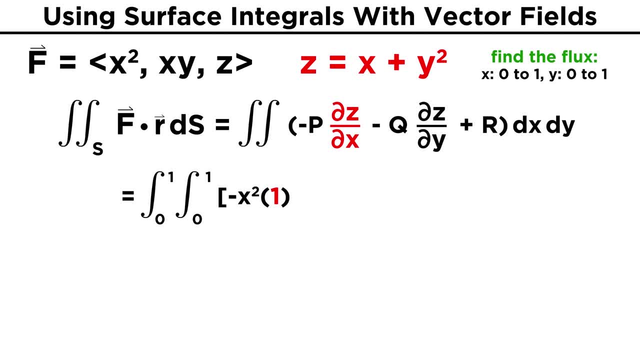 Remember which derivative The x plus y squared? I'm sorry, I'm thinking the 2x-elin diapers. Play your instrument, play your instrument, play your instrument. P plus y is x squared, so d, z, dy plus xx還是 x squared times z. 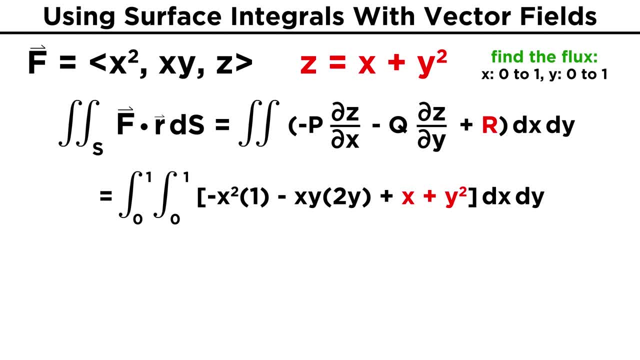 When you get this power sum, plug this in and this is y squared plus x and y squared. That's one plus y squared c RA. so this is 안녕하세요, this is two, this is three plus y-squared dxdy. 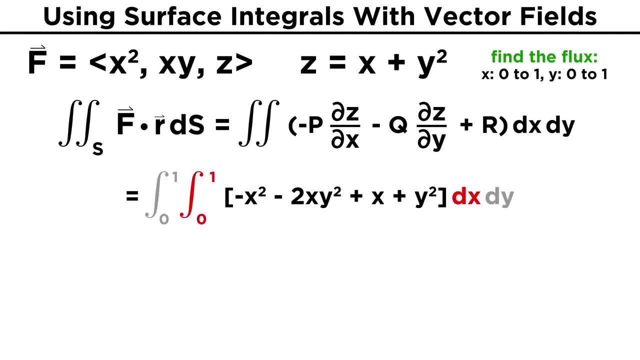 and y range from zero to one. Evaluating the x integral first, we get the antiderivative negative x cubed over three, minus x squared, y squared plus x squared over two, plus x, y squared, where x runs from zero to one. Evaluating at x equals one gives negative one third minus y squared plus one half plus. 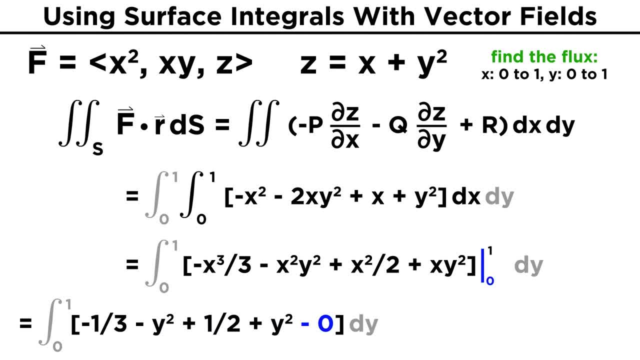 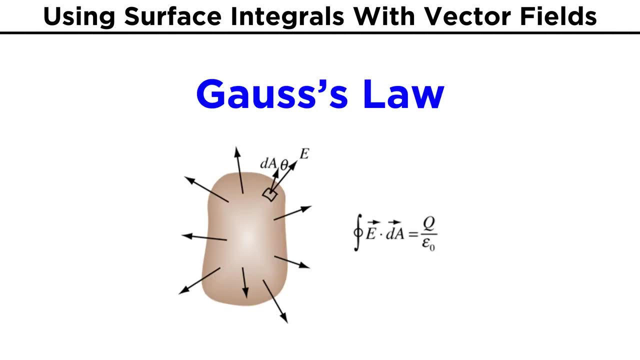 y squared while evaluating at zero will just give zero. The y squared terms cancel, leaving us with the integral from zero to one of one sixth dy. This gives us y over six, evaluated from zero to one, which is just one sixth. This will be our flux through this surface. 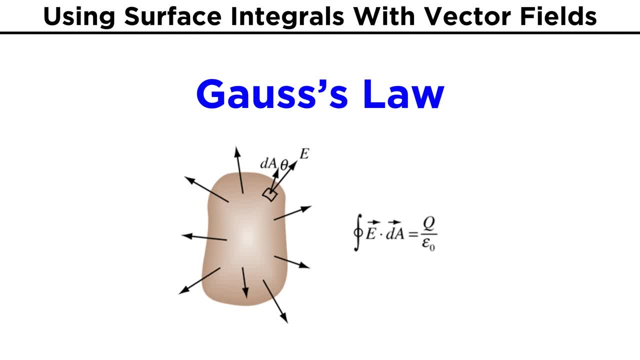 Surface integrals prove useful in many fields, such as when using Gauss's law in physics, which relates the amount of charge to the flux of an electric field through a closed surface. They are also used in some theorems which we will be discussing next. so with that in. 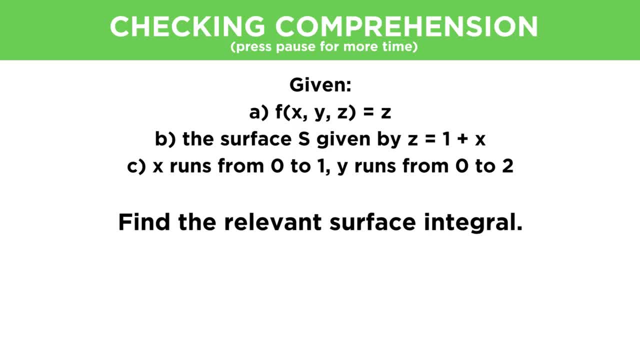 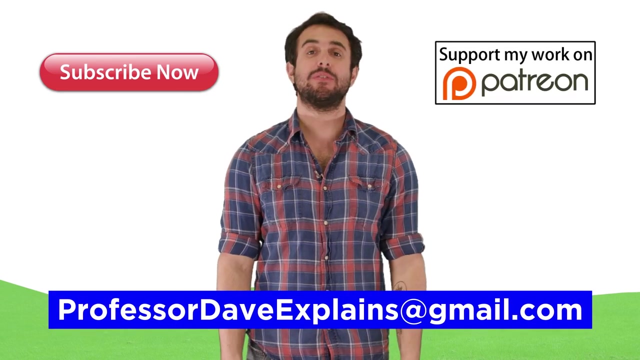 mind, let's check comprehension. Thanks for watching. guys, subscribe to my channel for more tutorials. support me on patreon so I can keep making content and, as always, feel free to email me professordaveexplains at gmail dot com. 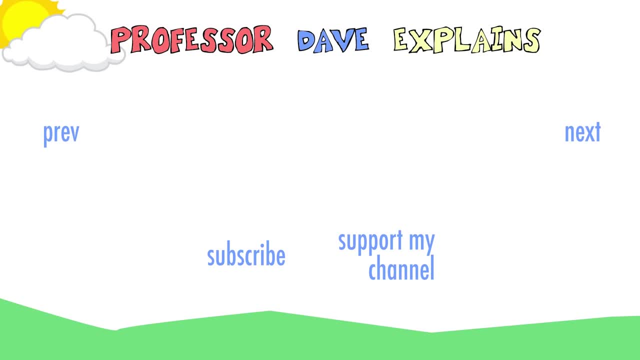 I'll see you in the next one.